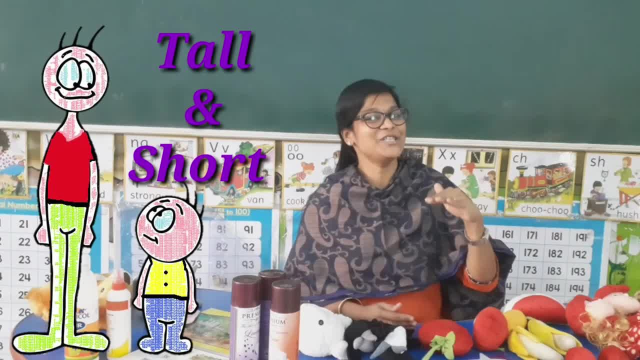 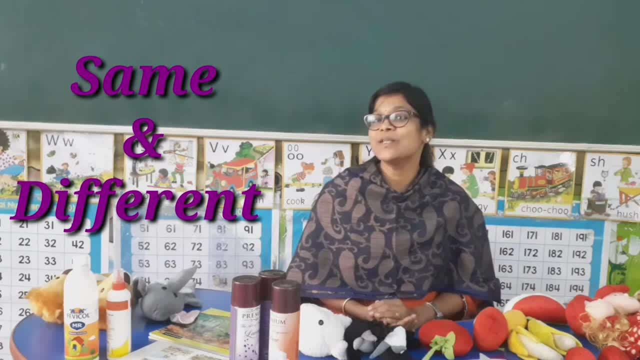 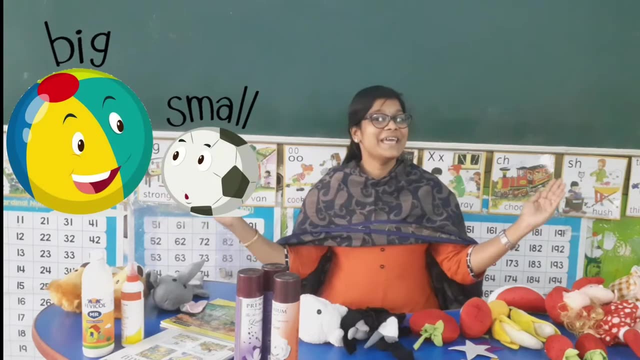 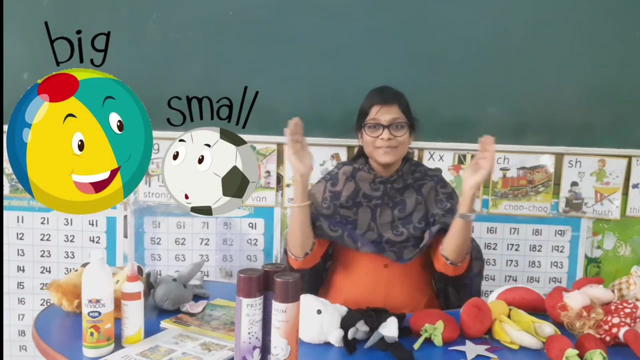 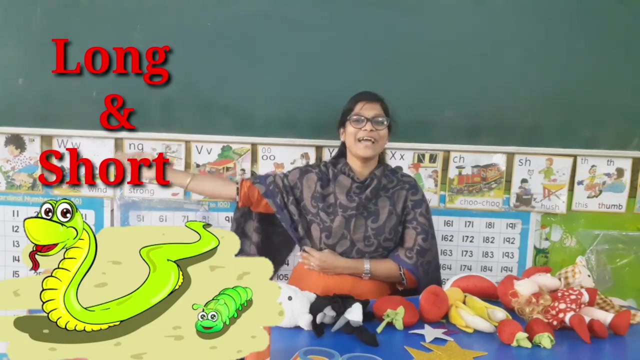 class ma'am taught you the concept all and short. For today we are going to learn the concept same and different. Before we move to our concept, let's sing the concept song. Come on, let's recall the previous concepts: Big, big, big, Small, small, small, Very good, Long and short. Long and short, Long. 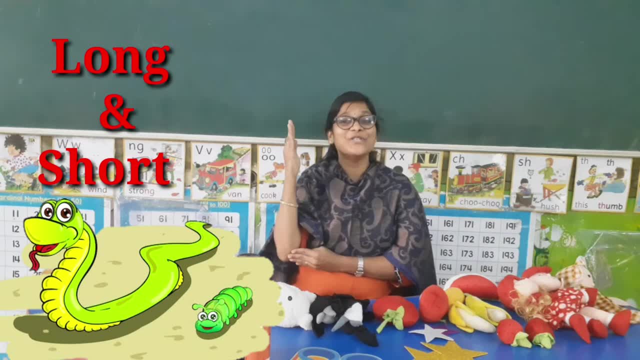 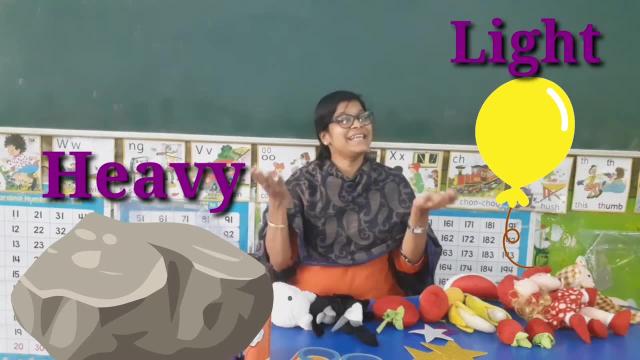 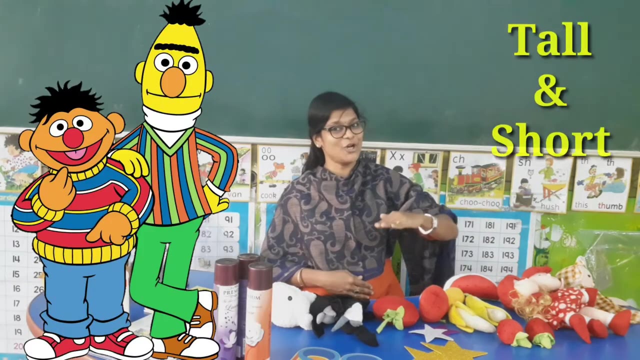 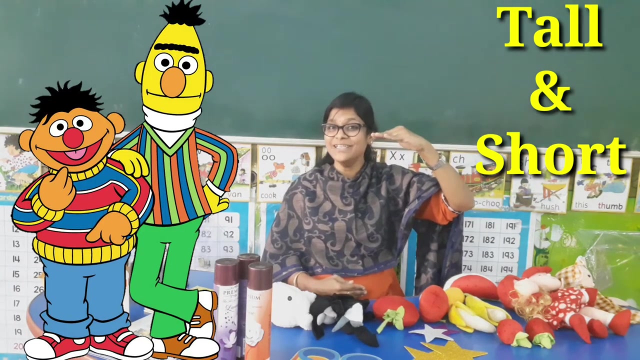 long, long, Short, short, short. Very good, What's the next concept? Heavy and light, Heavy and light, Heavy, heavy, heavy, Light, light, light. Tall and short. Tall and short. Tall, tall, tall, Short, short, short. For today, what are you going? 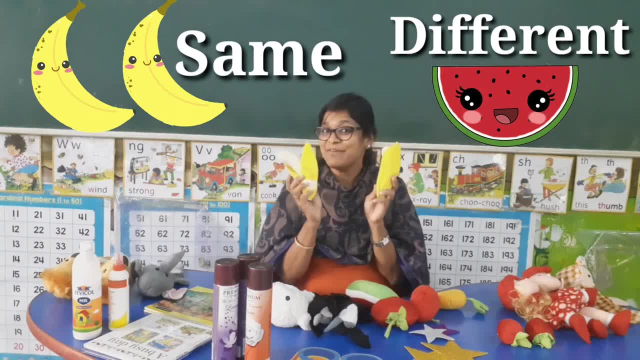 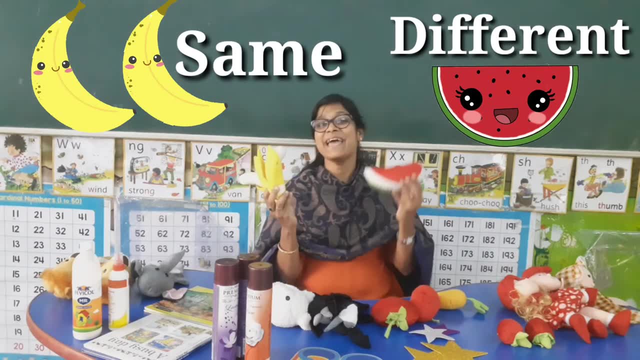 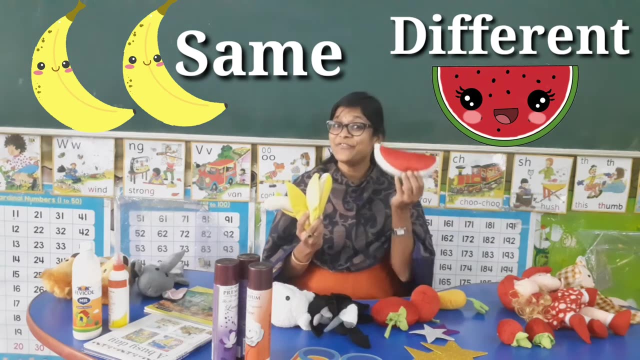 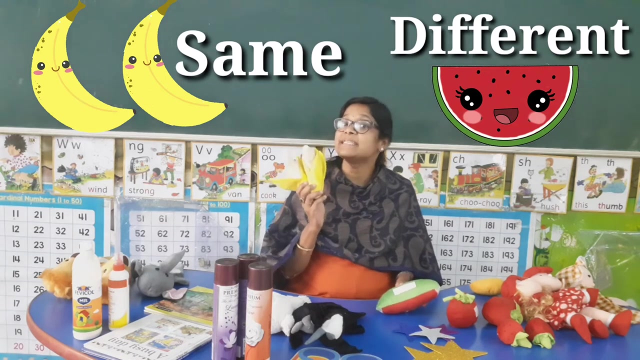 to learn The concept Same and different, Same and different. Same and different. Same, same, same, Different, different, different. Same and short, Tall, tall tall tall Short, tall, short tall. Same and different is classified by its size, colour and shape When they 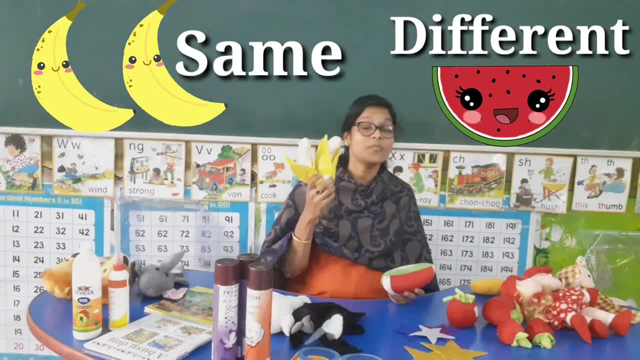 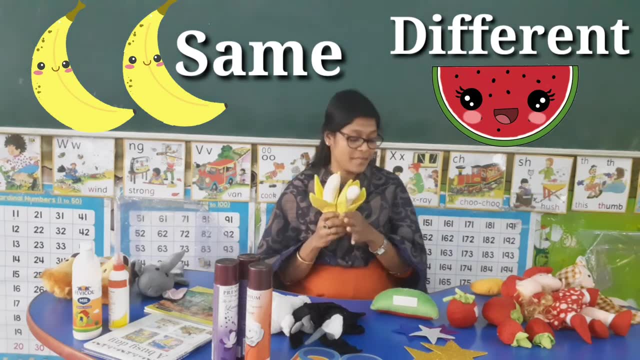 look the same size, colour and shape, we call it as same objects. It looks the same. we say it as same. When they do not look the same, we say it different. These two bananas are same. All of you see, tell me These two bananas are same. All of you see, tell me Whether. 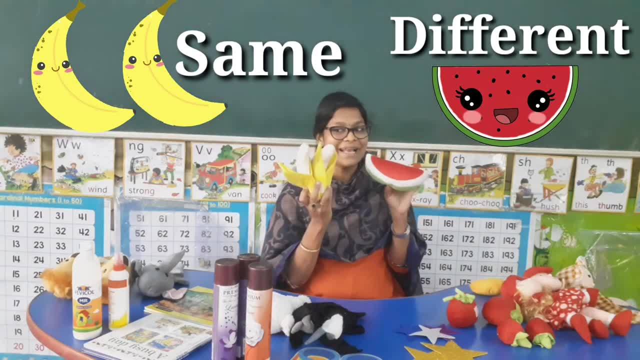 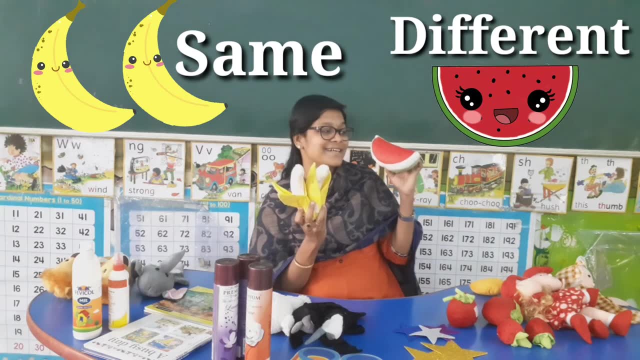 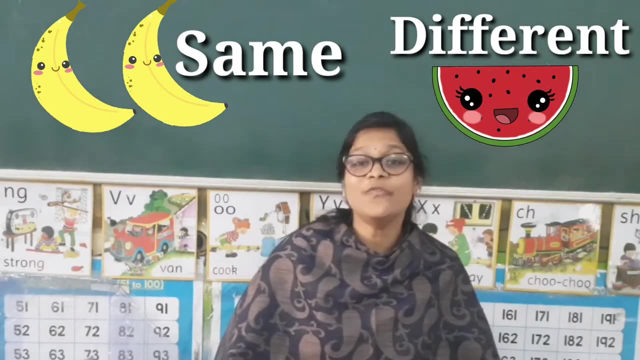 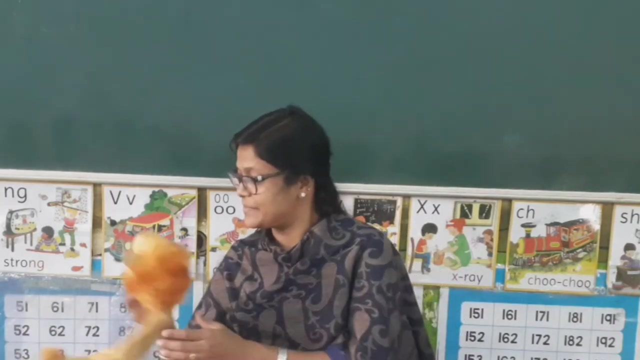 if you say same Compared to the banana, watermelon is different, How it is different, The shape is different and the color is different. Okay, my dear kids, Come on, let's move on to our lesson. I will show you few more examples for the concept same and different. Now see. 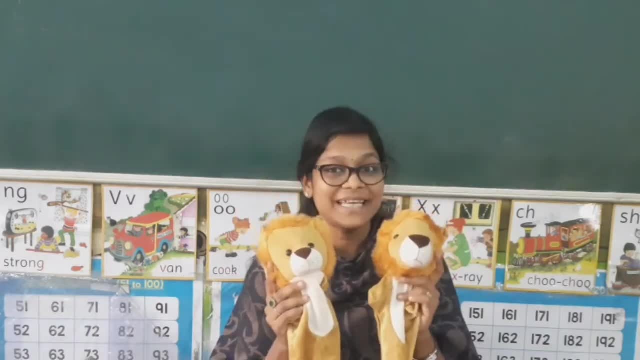 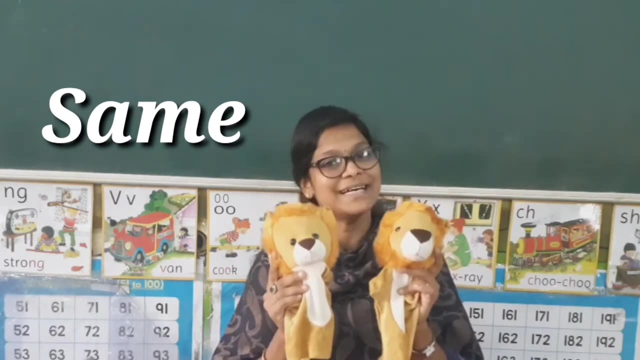 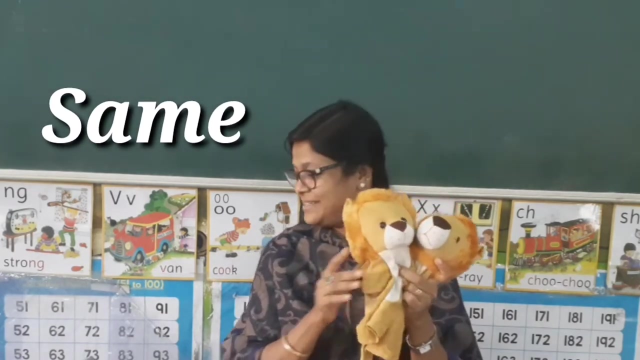 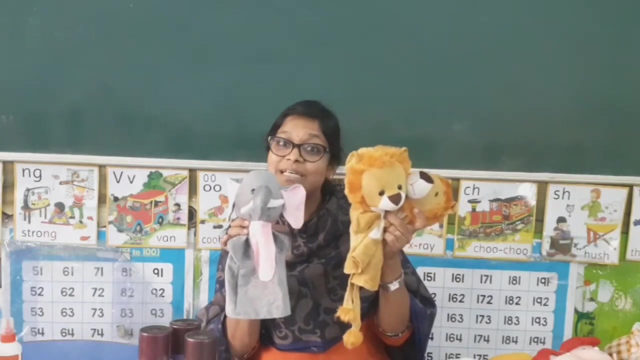 here. What is this? It's the lion puppet. The lion puppet looks the same. The lion puppets looks the same. All of you say same. All of you say, my dear kids, same. Very good, Now tell me, is the elephant puppet the same when compared to the lion puppets? No, it is different. 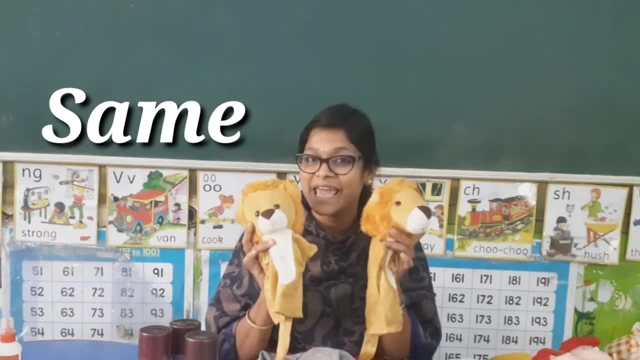 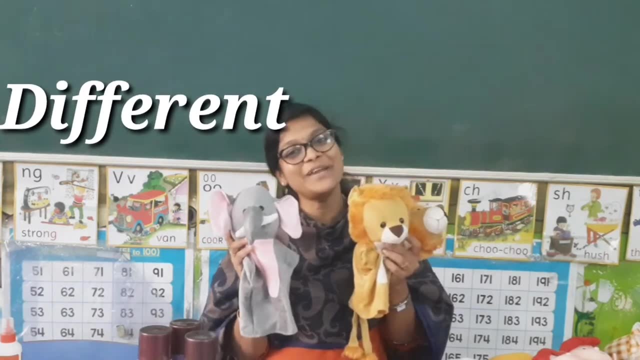 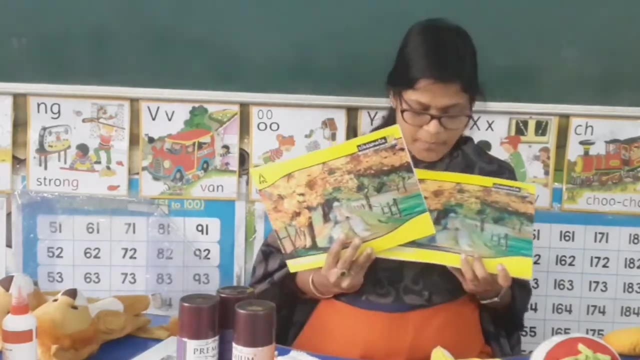 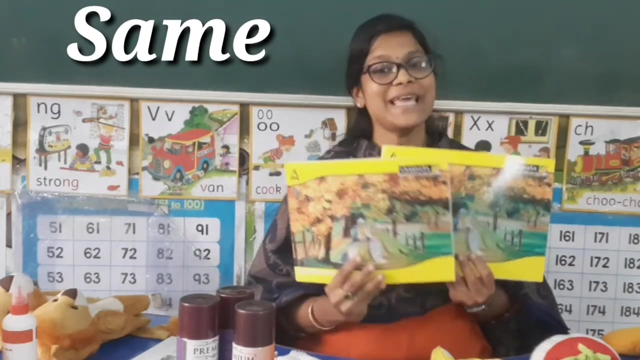 All of you say Different, Same, Different, Same, Different. Very good, kids, Very good. Come on, let's see the next example Now look at these two books. How many books I have One, two. These two books are same. All of you say same. These two books are same, Very good. 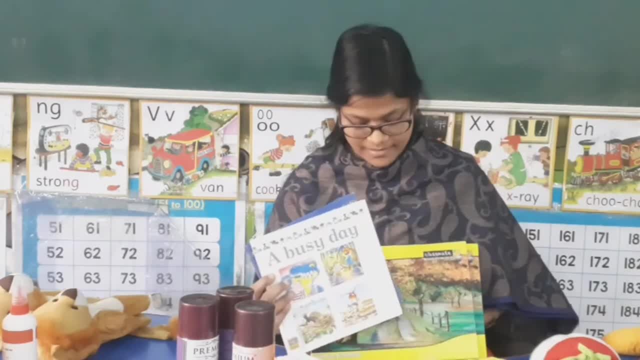 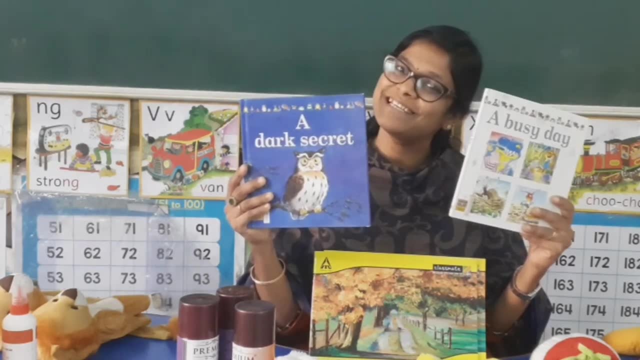 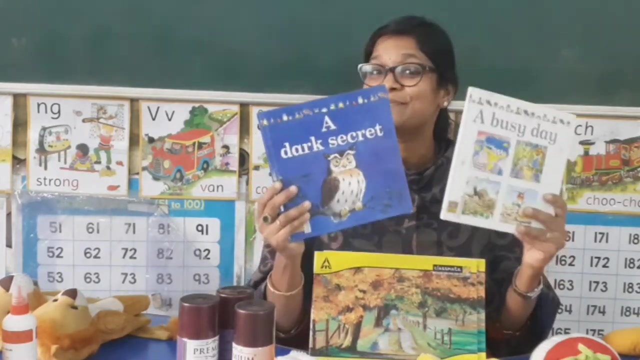 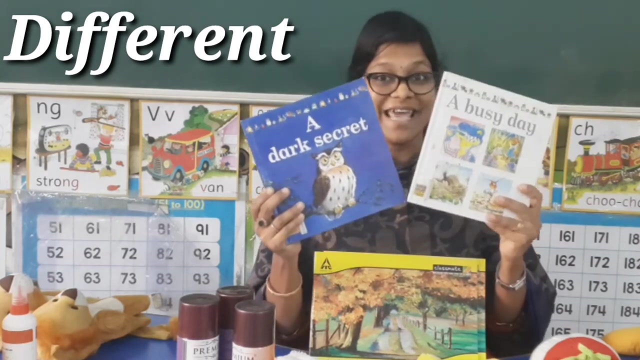 Now look at these books. Is these books are same or different? Tell me whether it is same or different. You are right, my dear kids. These books are different. How it is different, Different color, Yes, different. All of you say different. 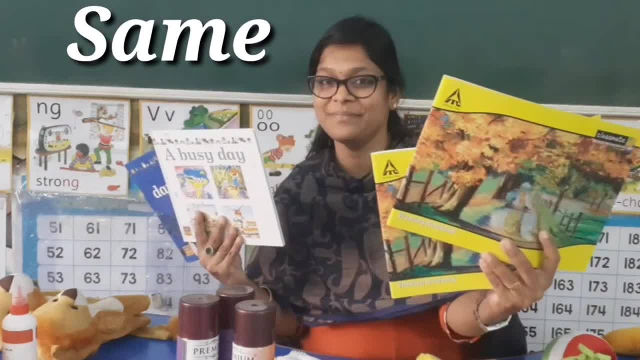 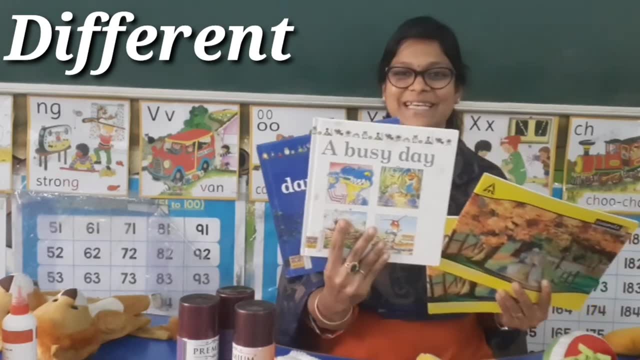 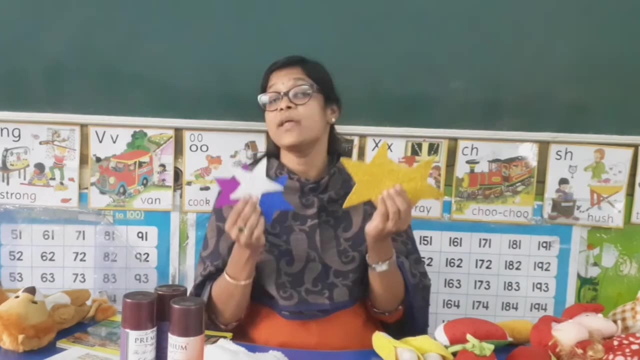 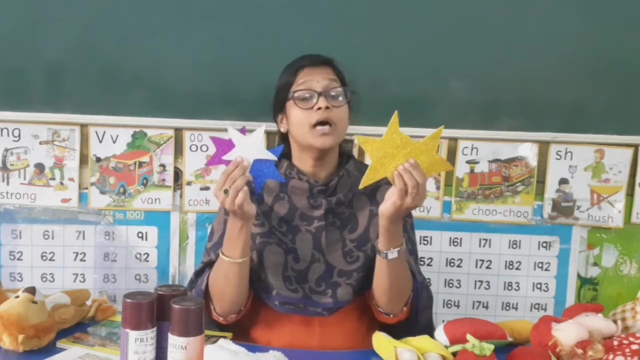 Same, Different, Same, Different. Very good kids, Come on, let's see the next example. Now it's your turn to find out which is same and which is different. Could you all see these stars, my dear kids? Tell me which stars look the same? Which star looks the same? 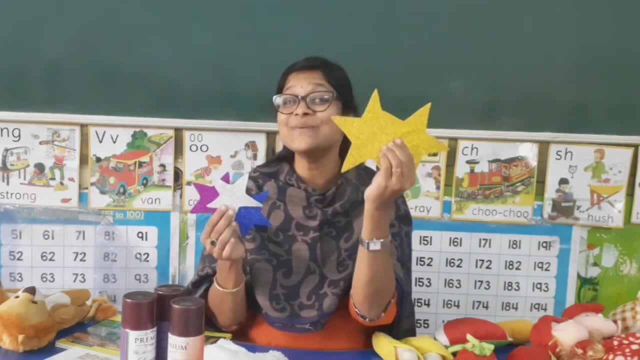 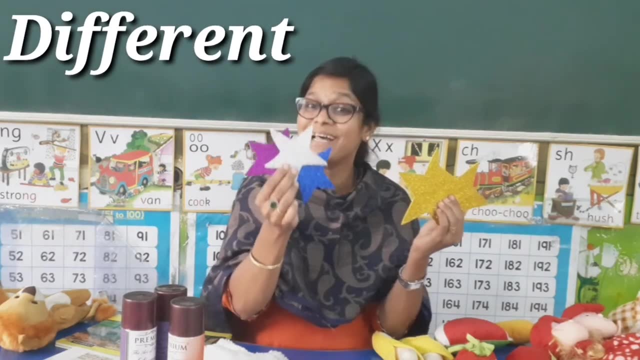 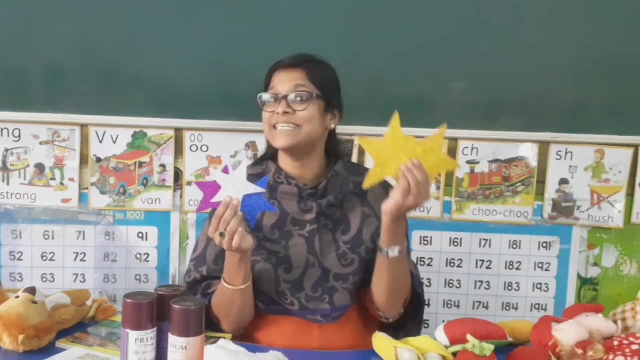 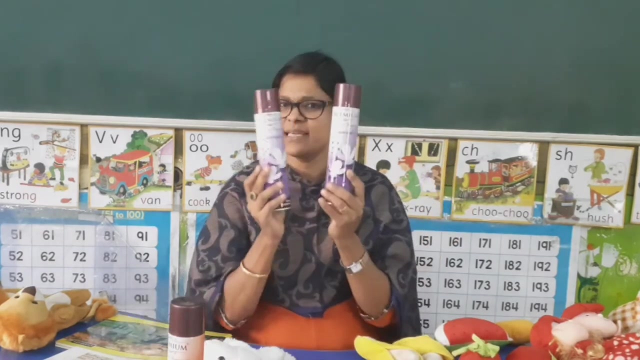 Very good kids, very good. Yellow stars looks the same And these stars looks different by color, Same, different. I hope you started to identify the same object and the different object. Come on, my dear kids, let's see the next example. Is this same? Is this same? 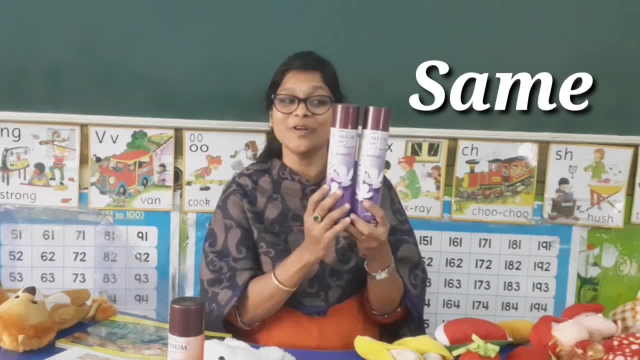 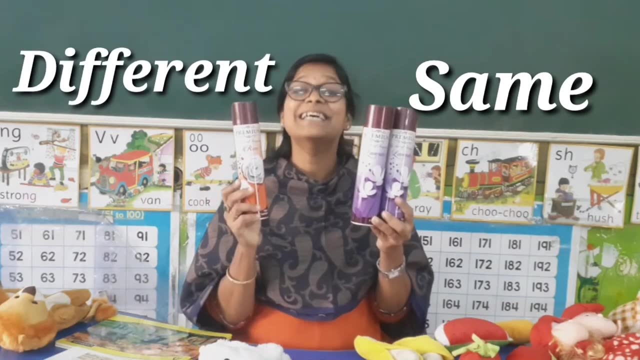 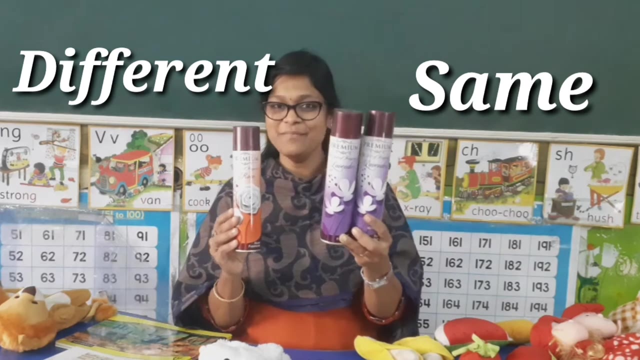 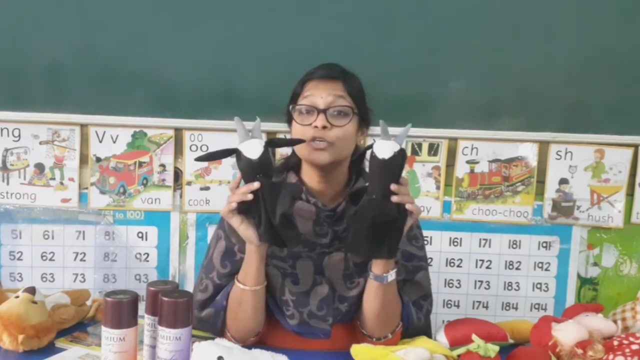 Yes, these bottles are same. All of you say same. very good, This is different, Very good. kids, same, different, Same, different, Very good, My dear kids now look at these puppets. What are these? Goat? it's a nanny goat. These two girls look the same. 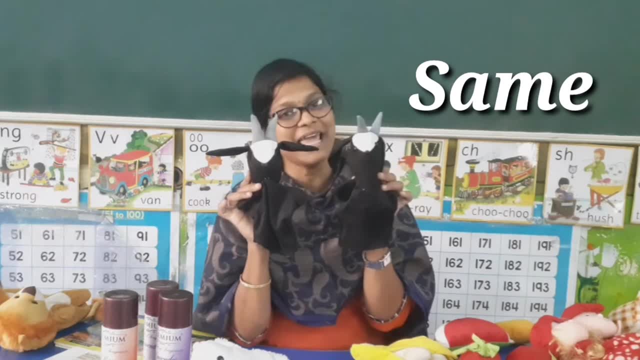 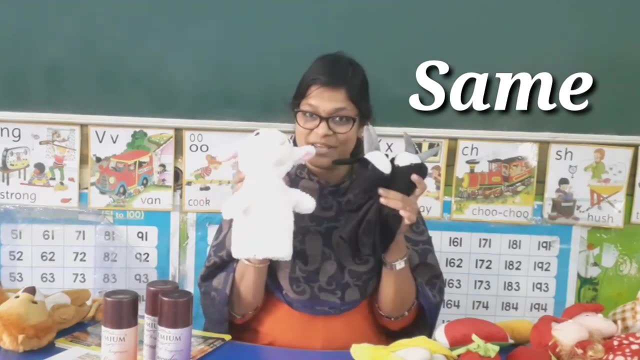 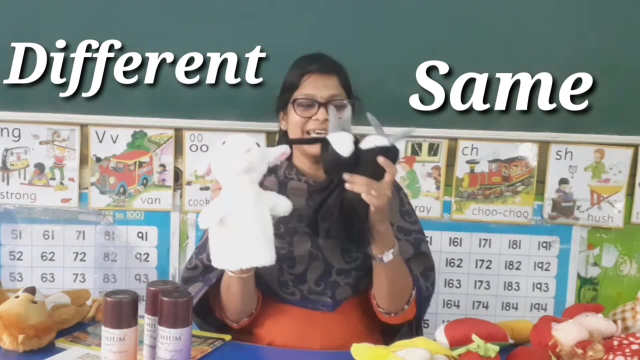 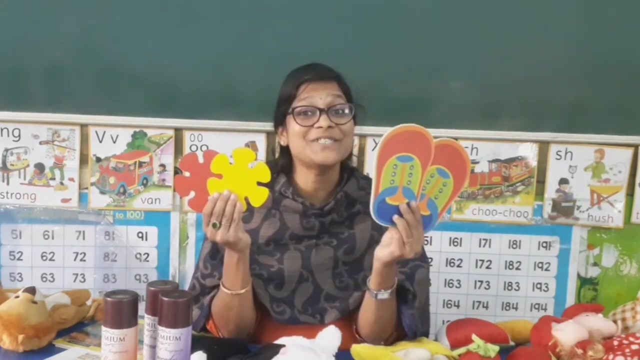 These two girls look the same. All of you say same, very good, Look at this sheep puppet. It is different when compared to this goat puppet. Different, same, different. Very good, kids. come on, Let's move on to our next example, These shapes, Which is same, my dear kids. 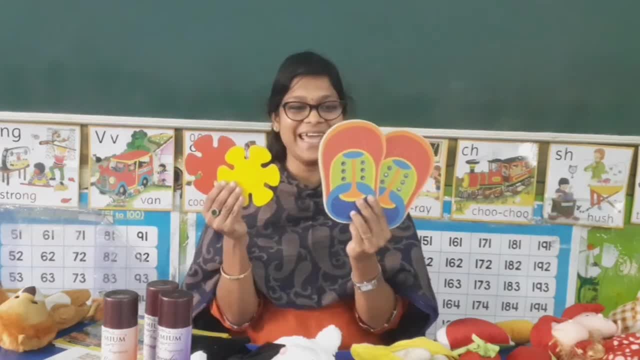 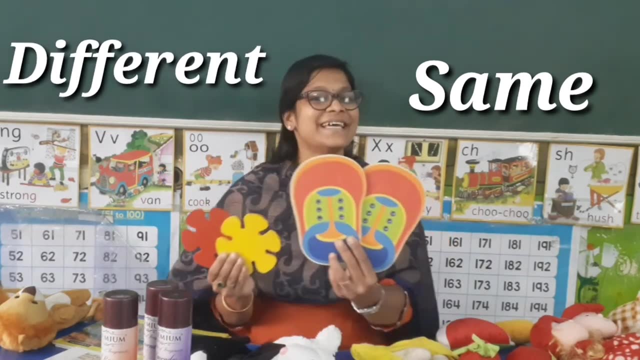 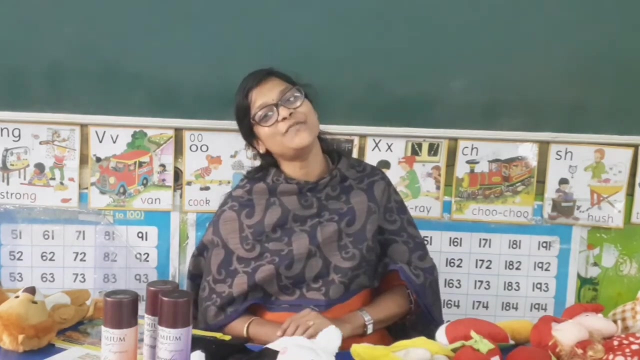 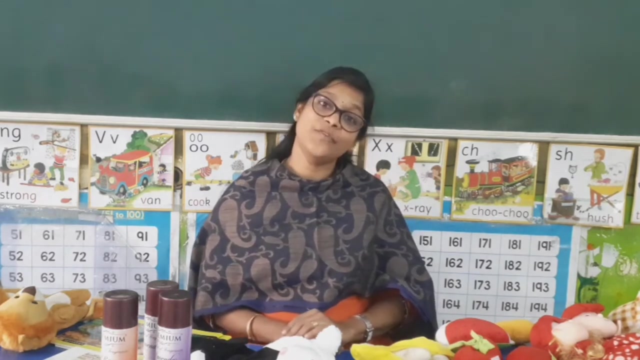 Could you identify Same? you are right, Same. all of you say same And this is different, Same, different. Very good, kids, very good. It's your turn to identify the objects which is same and different. I will show you few puppets and few pictures. 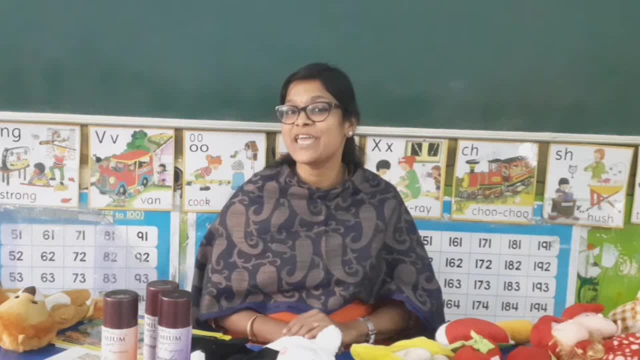 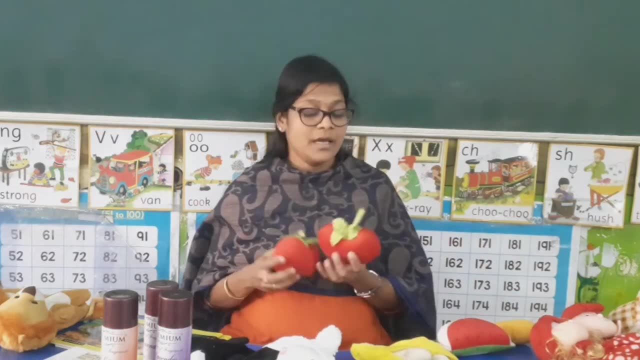 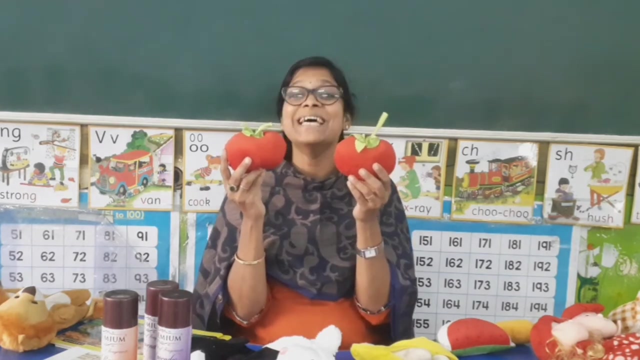 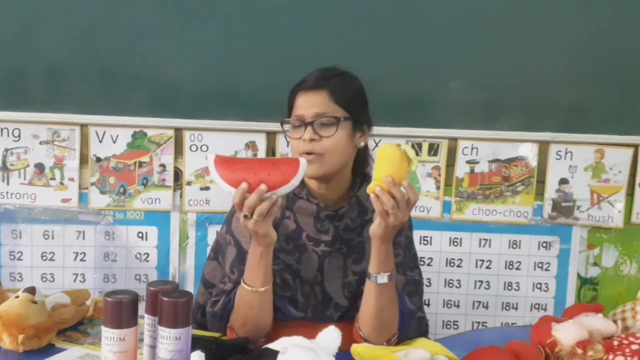 You should identify and tell me the same and different. Are you all ready, my dear kids? Okay, come on Now tell me, Is it same or different? Same, Same, very good kids, very good, Now tell me, is it same or different? Look at the puppets. 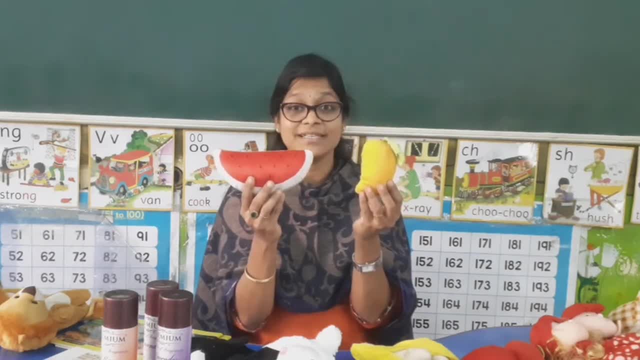 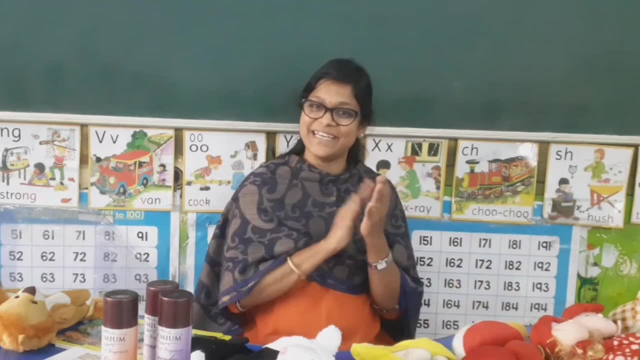 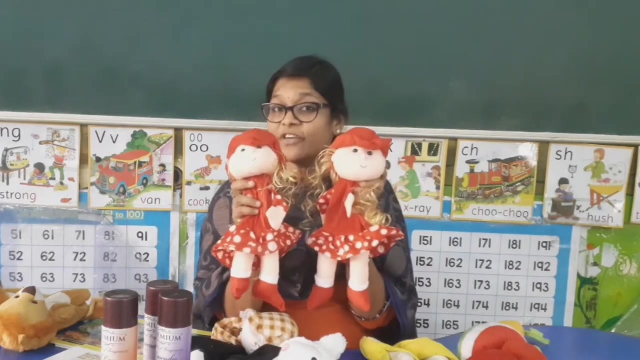 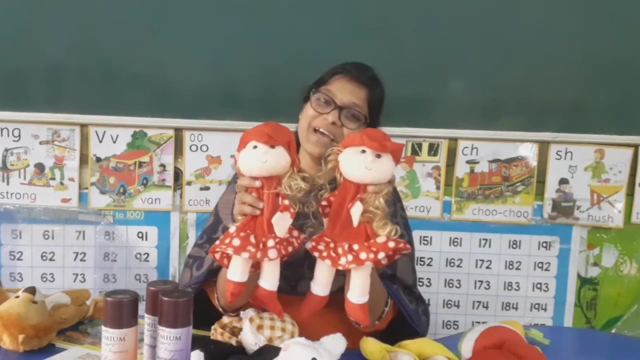 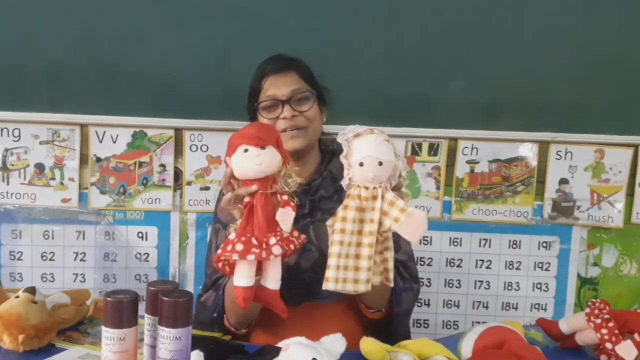 Tell me whether it is same or different. Different, Very good, it's different. Excellent kids, excellent, Very good. Now tell me whether these girls are same or different. Same, Yes, same. All of you say Same, Same, Same. Very good, kids, very good. Now tell me whether it is same or different. 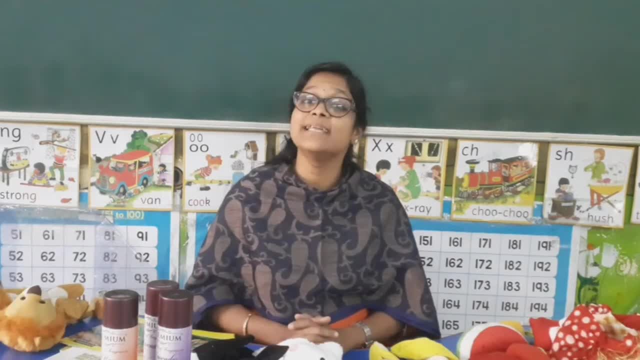 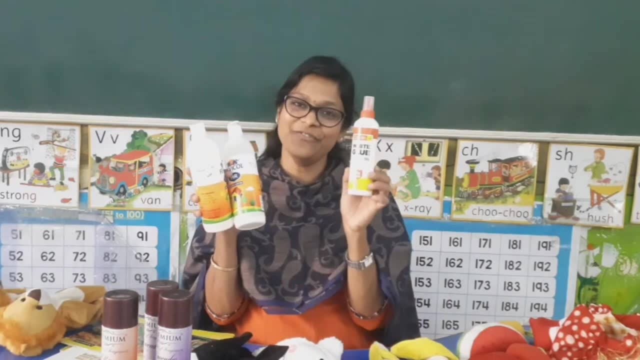 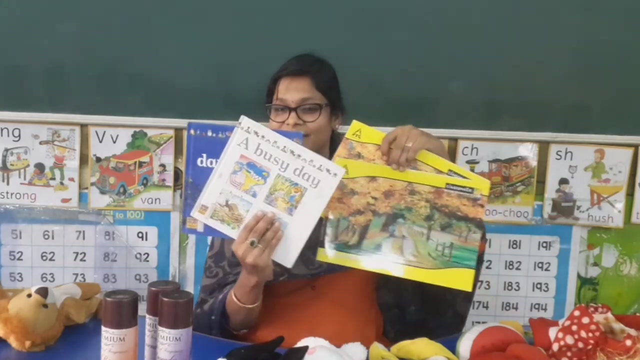 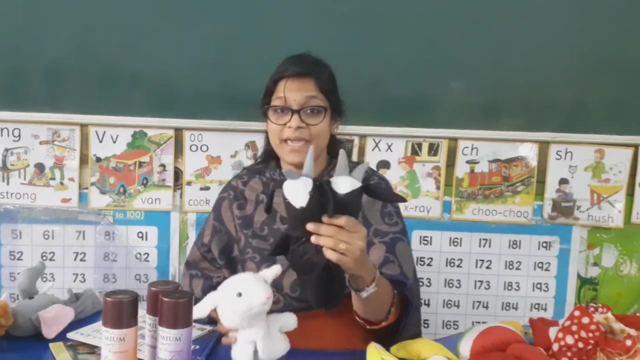 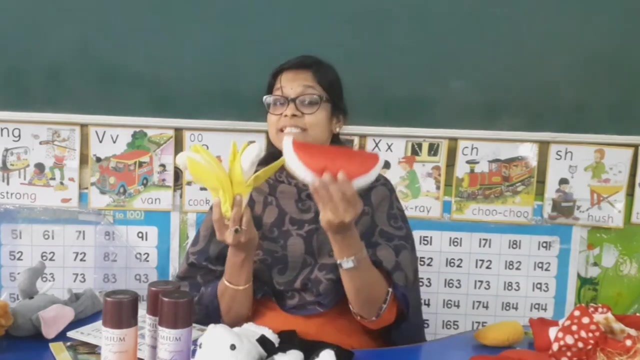 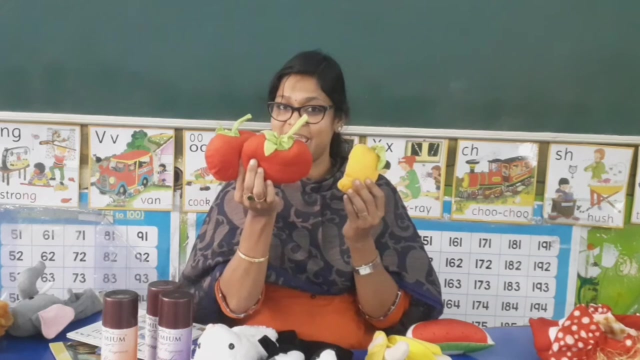 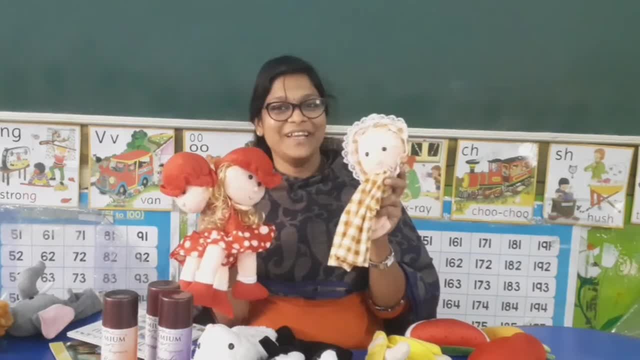 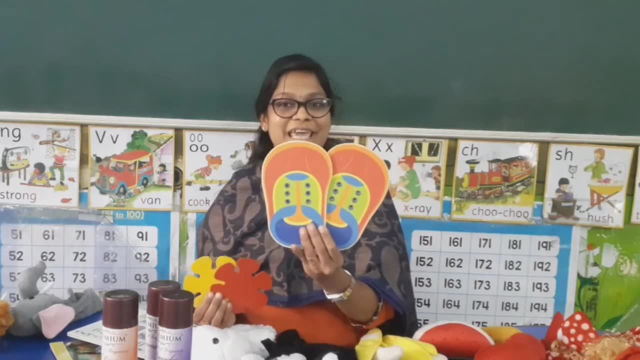 Same different, Same different, Same different.78 00 0000 000 03 мар שתratulations. आज तो उन्हों ले जान सकता है, कि खुशी की चल देख सकेगी. 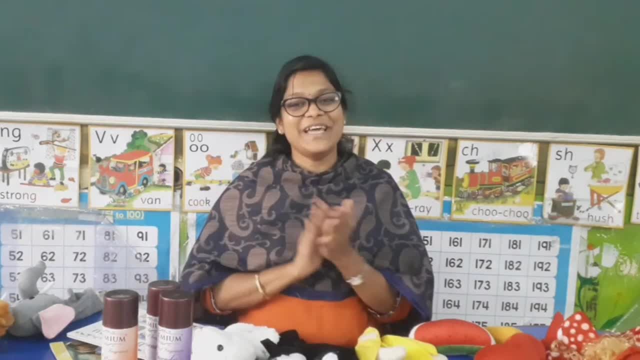 पौहाँत Angular सेखने खंवच सेखने ढिस्डologist: See different, Let's try See different, Let's see different, different. Thank you, kids. Very good, Very good. I hope you understood the concept same. 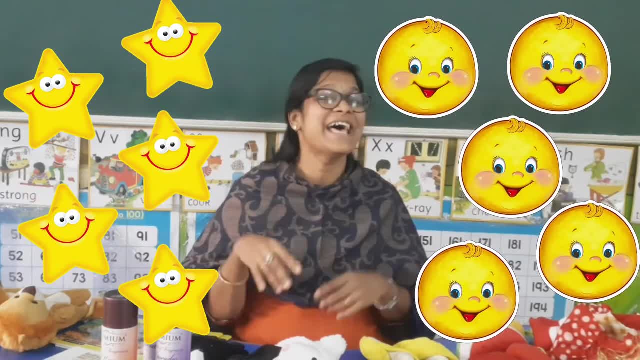 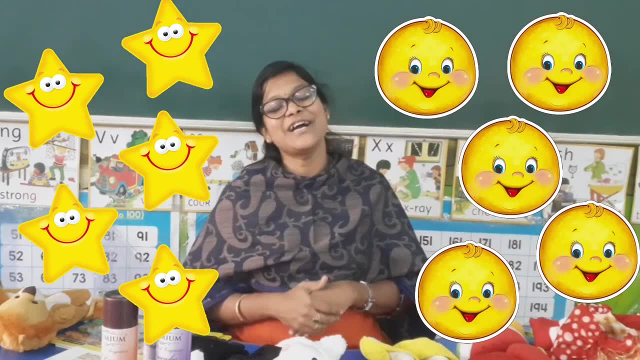 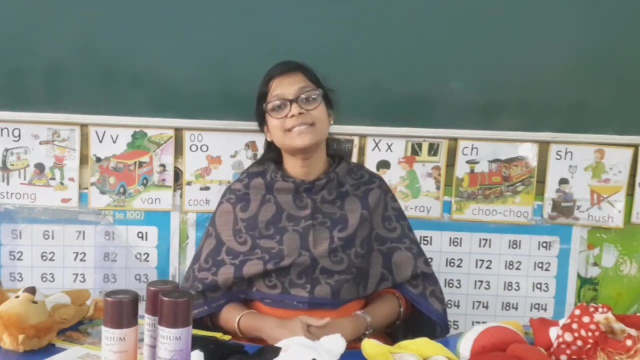 and different. Ma'am is giving you 5 stars and 5 smileys for understanding the concept same and different. Come on, let's see some more examples. I will display few pictures. You can look at these pictures and identify whether it is same or different. Same- different. 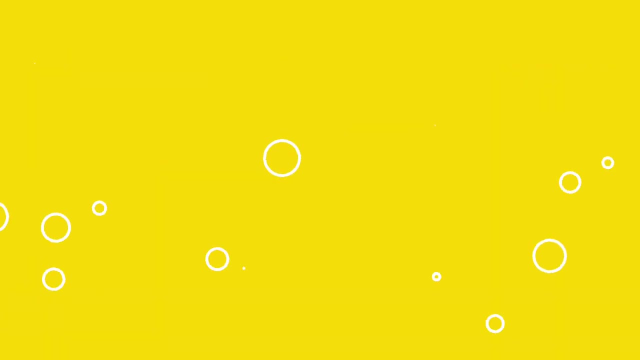 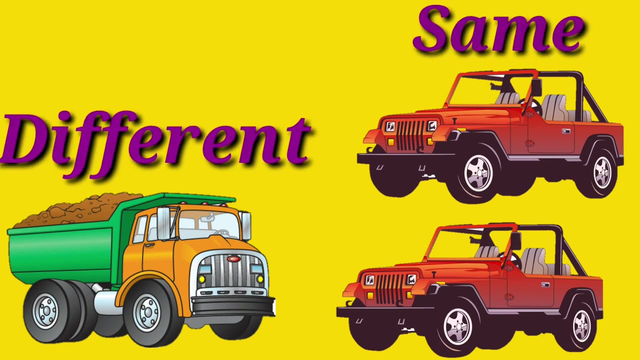 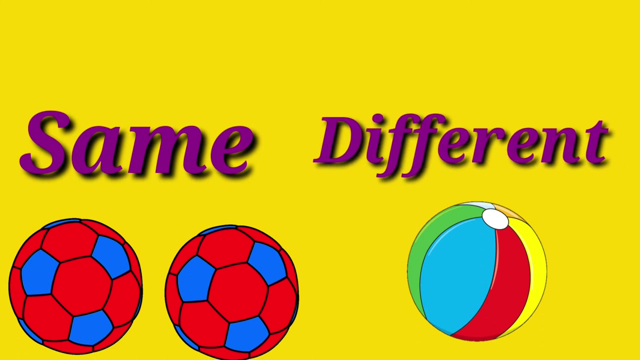 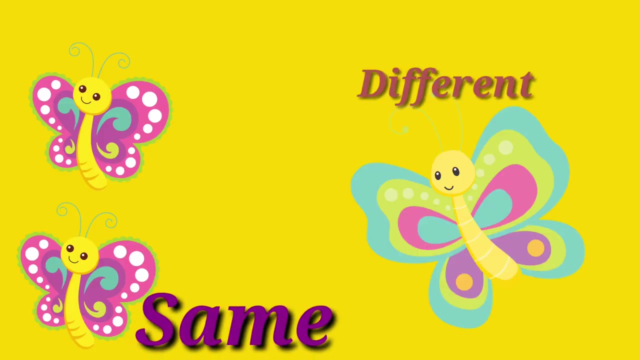 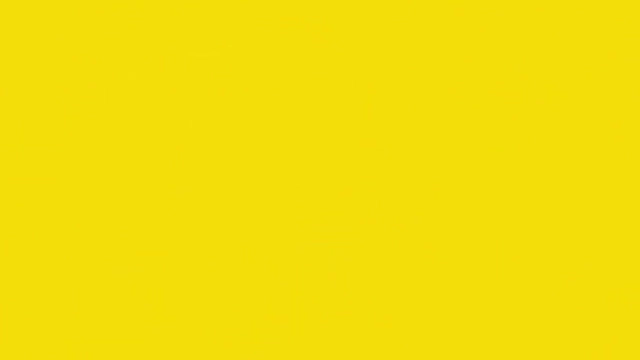 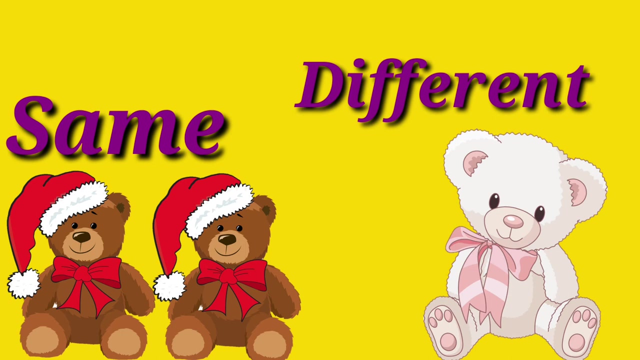 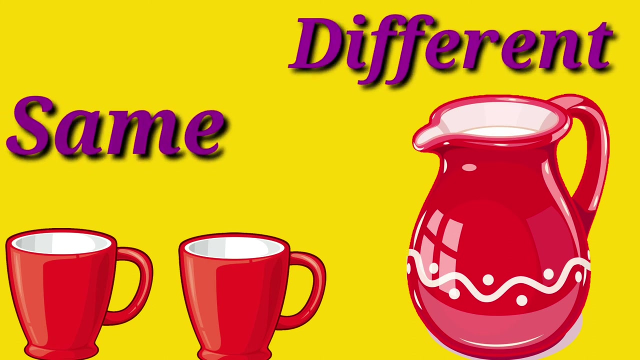 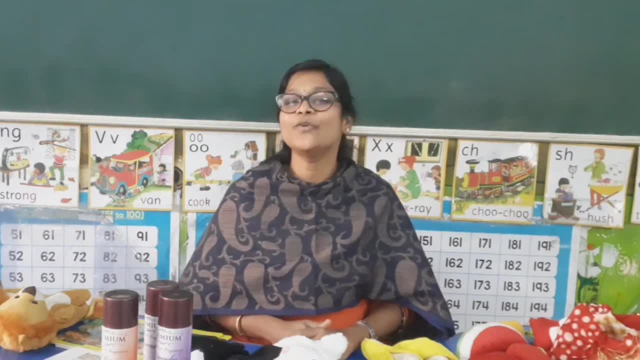 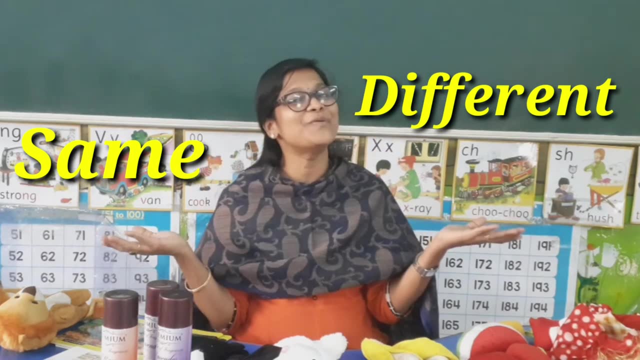 What are you going to do At home? you are going to collect few objects or few things, which is same and different. You are going to take a video and post it to math. Will all of you do it, my dear kids? Very good, very good kids.